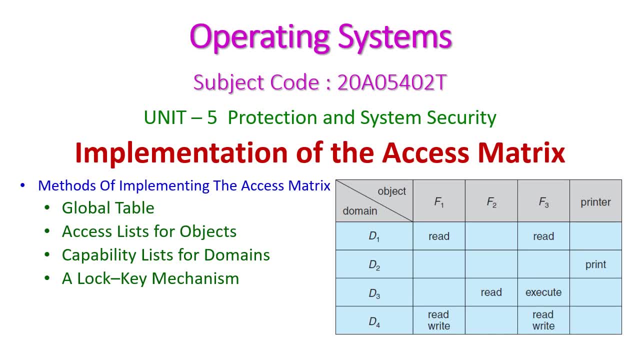 Hello friends, in this operating system class we will see the second part of access matrix, that is, implementation of access matrix. Here there are four methods to implement this access matrix. First one is global table: access list of objects, capability list of domains and lock key mechanism. Let us see all those things one by one. 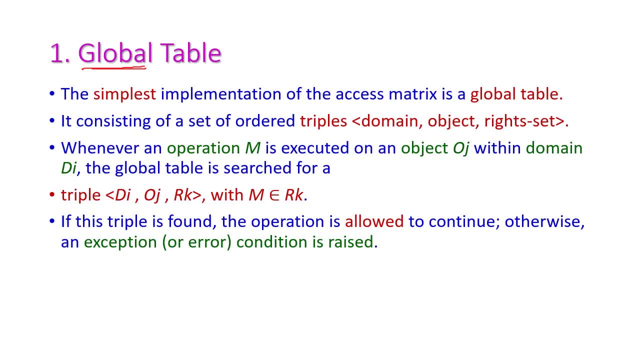 The first implementation model is global table. This is the very simplest one and it consists of order triples, which contains domain object and a right set, that is access right set. Whenever an operation is executed, this particular object within this domain, then the global table is searched for this triple, that is domain object and access right. 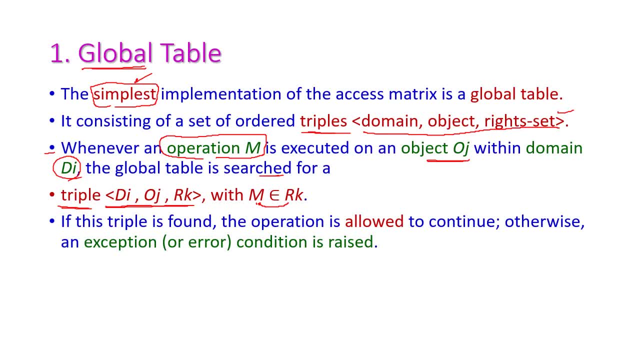 Okay, and the operation should be: belongs to this access right, that is, it should be access for this particular right. on the object: Okay, if the triple is found, then the operation is allowed to continue. otherwise, the exception condition is right. that is the error message will be given for the user. 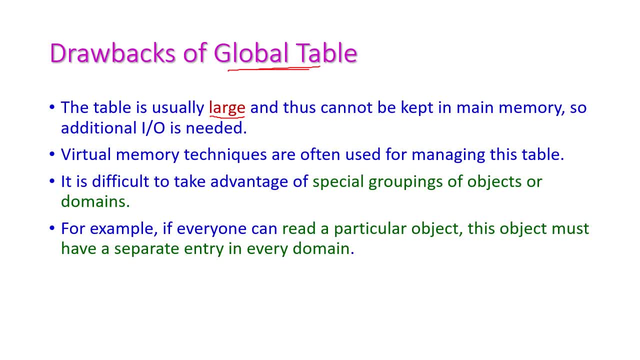 Next, let us see the drawback of global table. The global table is very large in size. So we can see, the global table is very large in size, cannot accommodate that table in the main memory. hence it required additional I, O, that is, input, output or secondary storage devices. right, and hence we have to implement this. 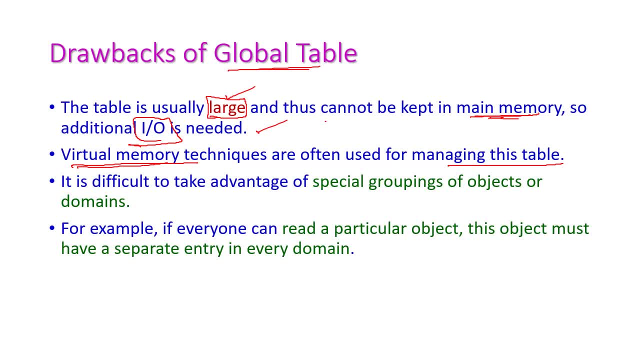 virtual memory technique to manage this very large size global table, because the size is very high. so we have to implement this virtual memory technique and it is difficult to take advantage of special grouping of objects or domains. and we can see one example for this: if anyone read a particular object, anyone read a particular object. this object must have separate 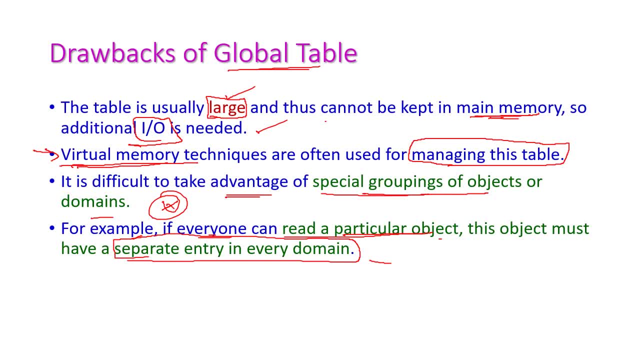 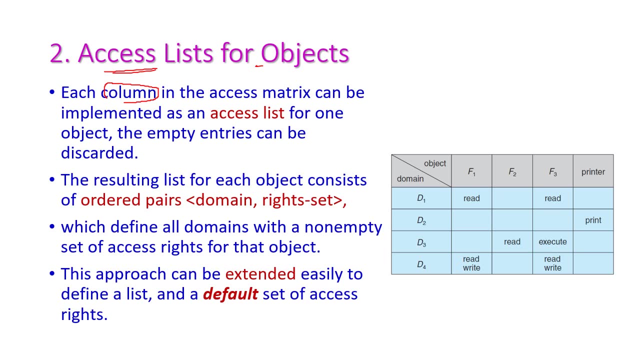 entry in every domain, so that the size will get very much increased for this global table, and managing and maintaining this global table is very difficult. the second one is access list for objects. here each column in the access matrix be an implementer as access lists for the one particular object. for example, and this is the access list for this particular. 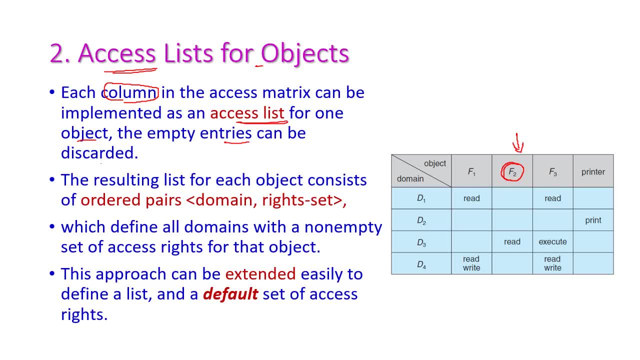 object. here, empty entries can be discarded. see, these are empty entries. this can be discarded. right, and the resulting list for each object consisting of: ordered pair of the domain: commit: right. ordered pair of domain- comma- right, okay, see, this is domain and this is the corresponding right of this particular object, which means that define it defines all domains with non-empty sets. 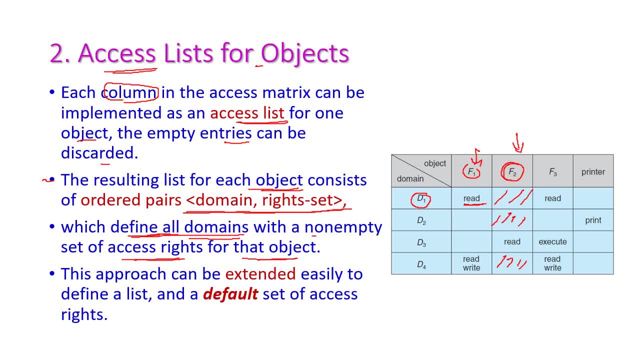 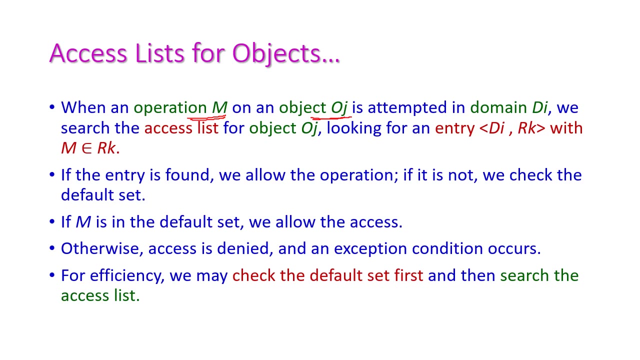 of access right for that particular object that is in domain d1. the file f1 is having only read access. okay, this approach can be extended easily to define a list and a default set of access right. when an operation m on the object j attempt in domain d i, domain d i, we search the access list. 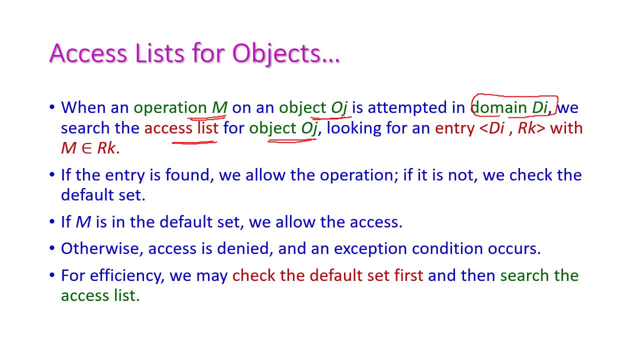 for object oj and looking for entry d i comma r, k d i m. on the object b j attempt in domain d i, we search the access list for object o j and looking for entry d i comma r k d i means to define a list for object o j and for the existing. 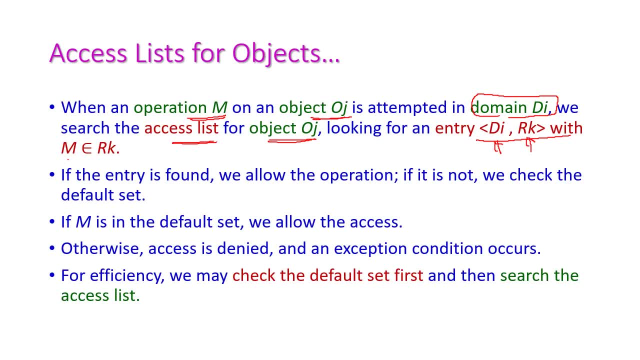 means domain, rk means access. with the m- m means operation, operation should be accessed, this particular right, okay. so we need to test whether in this particular domain, which access is given for that particular object, for particular object. so we need to test that in the access matrix. if entry is found, then we allow that particular operation to perform. otherwise. 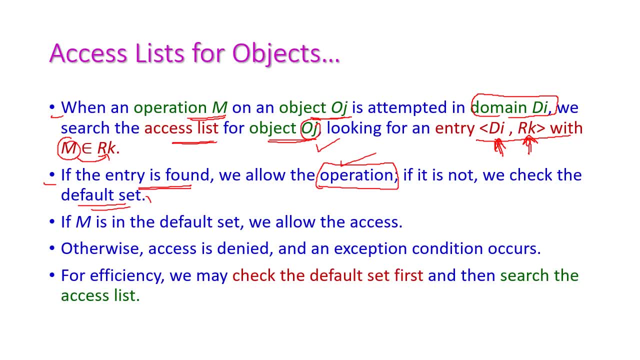 we have to check the default set list, and if m is in the default set, then we can allow the access. otherwise the exception will occur, that is, error message will be raised. for efficiency, we may check the default set first and then search the access list, so so that we can. 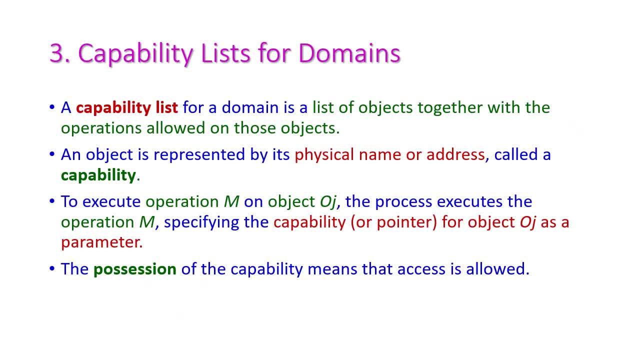 reduce the access time. the third one is capability list of domains. capability list for a domain is a list of objects together with the operations allowed for those objects. okay, capability list which contains objects along with the operations, right and the object is represented by the physical name or address. 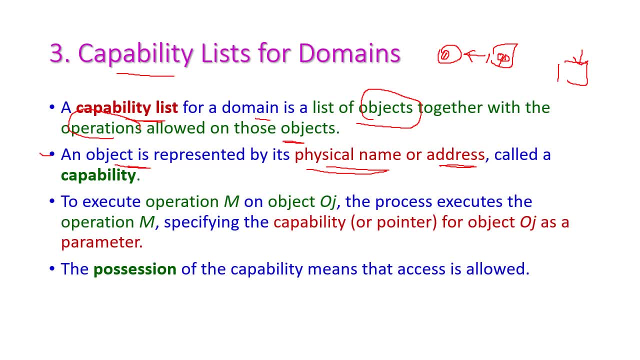 okay, in the memory where the object is exactly stored and which is called as capability, and to execute an operation on this particular object. okay, the process executes the operation specifying the capability for the object as a parameter. okay, so for executing this particular operation, we have to give the address of object. 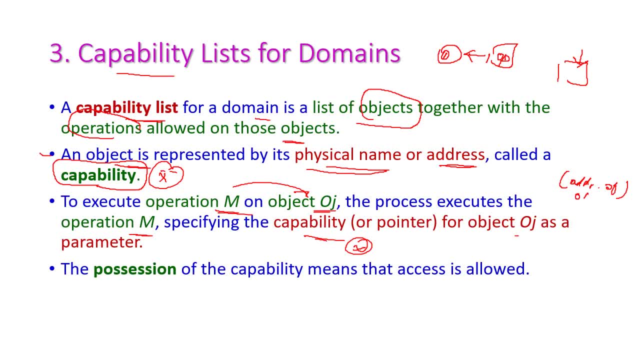 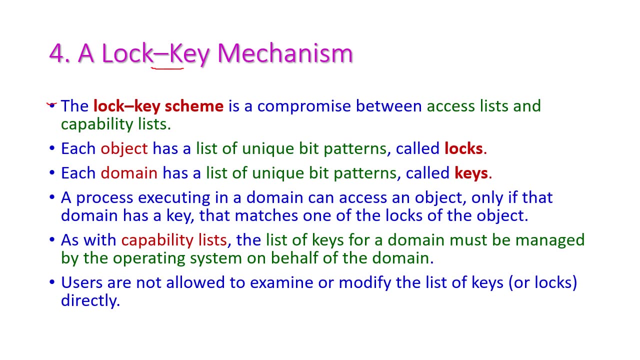 okay, address of object as the parameter right and the position of capability means the access is allowed. the fourth one is lock and key mechanism. okay, and it compromise the access list and the capability list. okay, in this lock and key mechanism, each object has a list of unique. 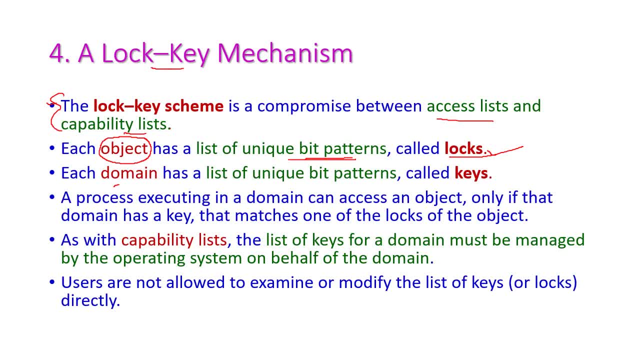 bit pattern, which is called as locks, and each domain has a list of unique bit pattern that is called as key. hence it is called as lock and key mechanism. okay, suppose if you want to execute a particular process and in your domain, then it can access an object, isn't it only if the domain key should match with?